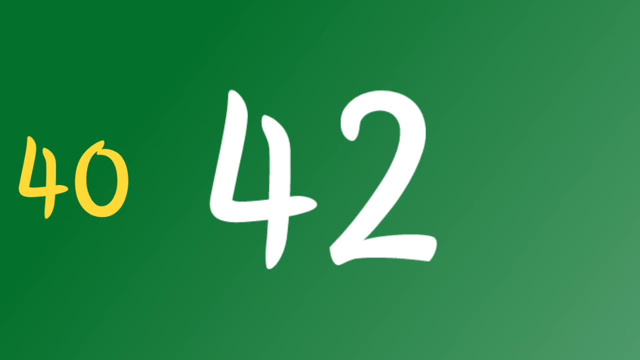 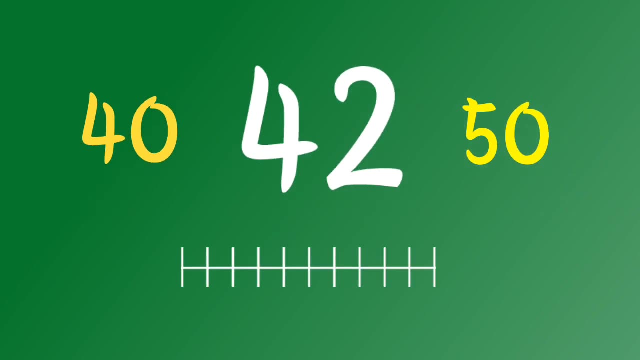 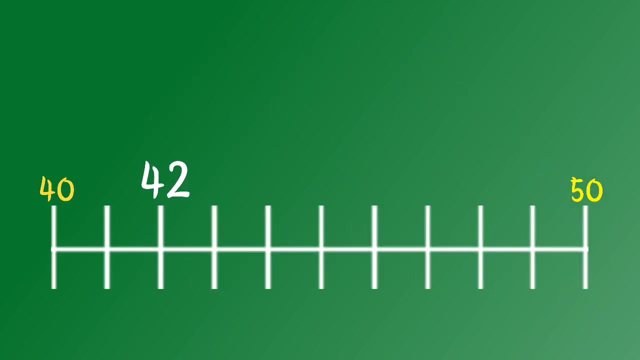 number of 42, 40 or is it 50? using a number line, you can easily decide a rounded number of 42. see the nearest round number of 42. is it 50 or is it 40? it is based on the nearest round number, so it's 40. so what if it's 45? in this case, we'll 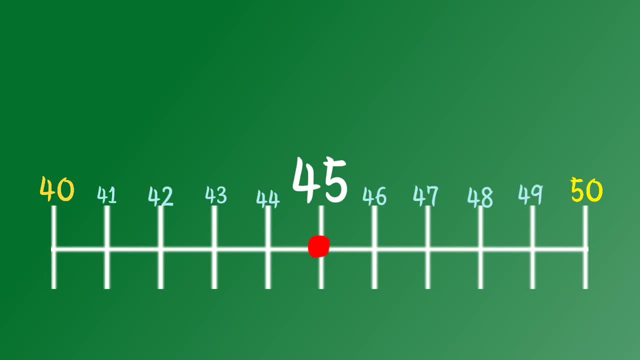 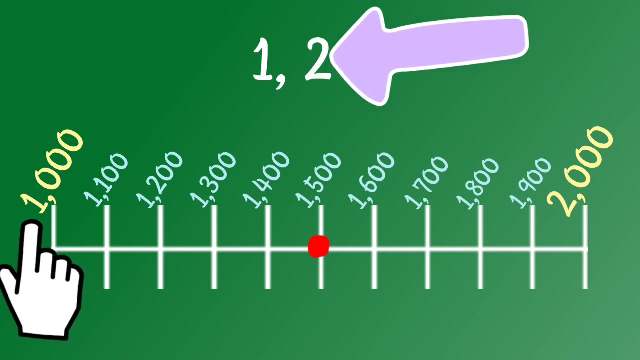 go with a round number with the highest value, so it's 50. let's try the number of seedlings in the number line. where can you find one thousand two hundred ninety three? okay, let's search. so somewhere here. one thousand two hundred ninety three is somewhere here. 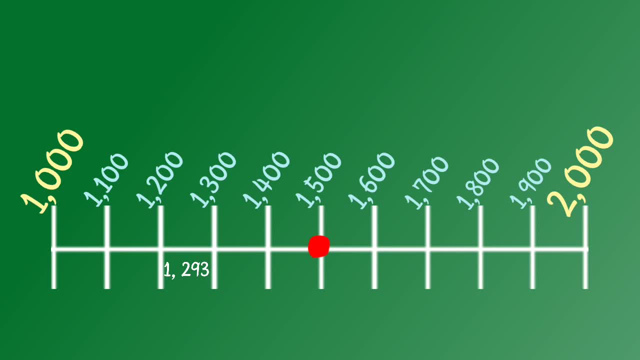 again, it is based on what round number is nearest to one thousand two hundred ninety three. so if 1293 is here, it's nearer to 1000 compared to 2000.. the rounded number of 1 293 is 1000.. Try 1632. 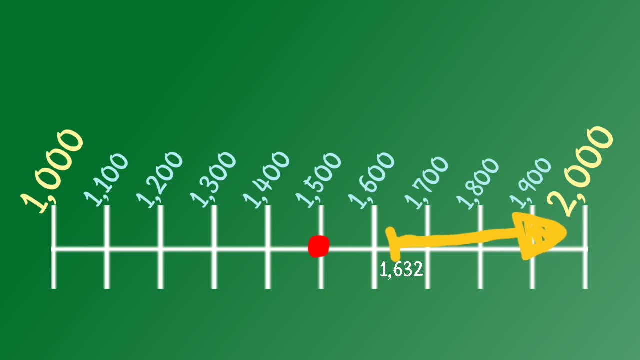 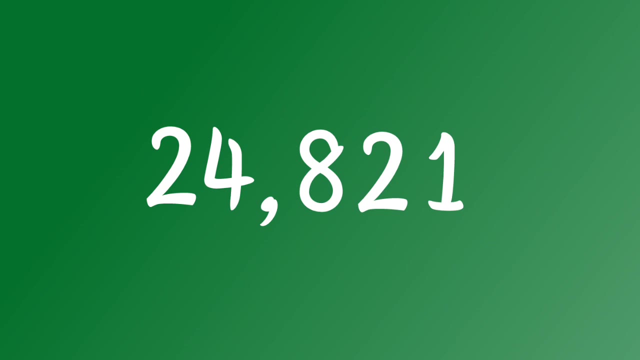 So the rounded number of 1632 is 2000.. Okay then it's time to learn the procedure we follow to round off a number. In this part, we have to remember the place value of a digit in a number. Let's say, for example: round this number to the nearest thousands. 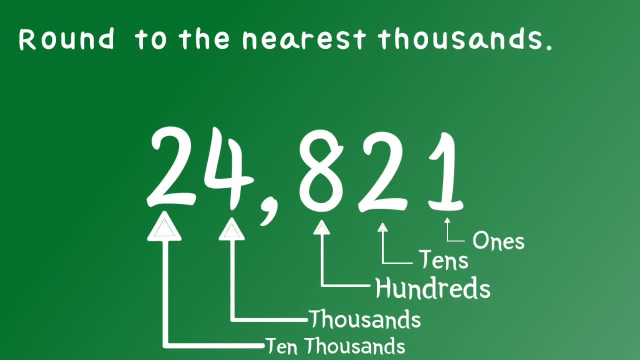 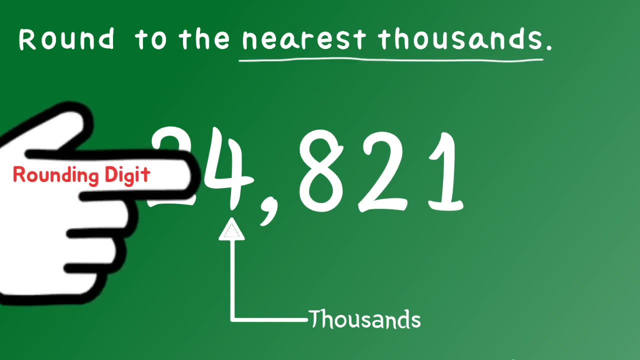 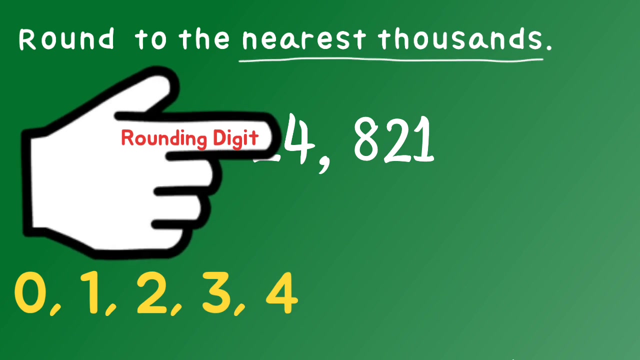 Nearest thousands. Four is in the thousands place, So four is the rounding digit. No need to use the number line to decide whether 24,821 will become 25,000 or 24,000.. Just remember when the next digit at the right of the rounding number is less than. 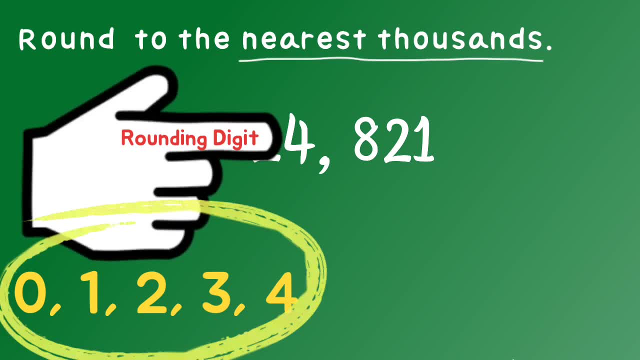 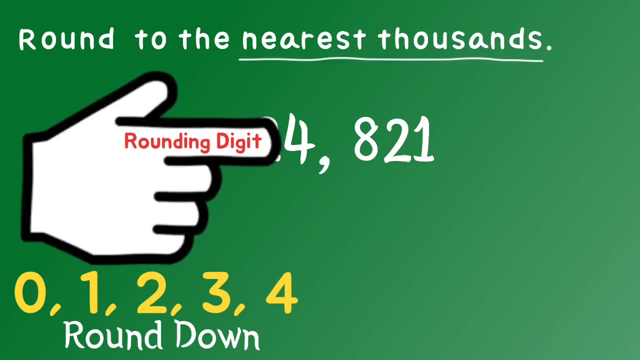 5, like these numbers, then we have two round down, Meaning This four here will remain as four. But when the next digit at the right of the rounding digit is either five or more than five, like these numbers, then we have to round up by adding one to the rounding digit. 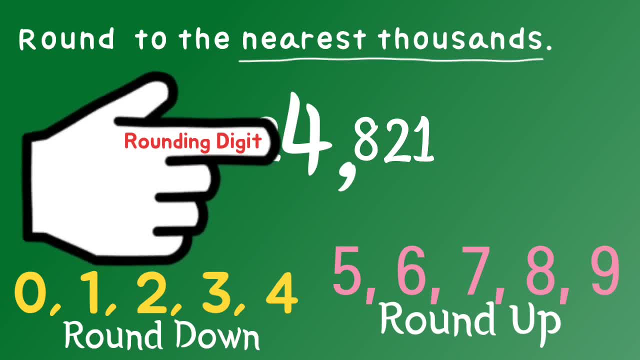 To make it clearer, here's your rounding digit. When this digit to the right of your rounding digit is either 0,, 1,, 2,, 3, or 4, the rounding digit will remain as four. But if this digit is less than five, then we have to round up by adding one to the rounding. 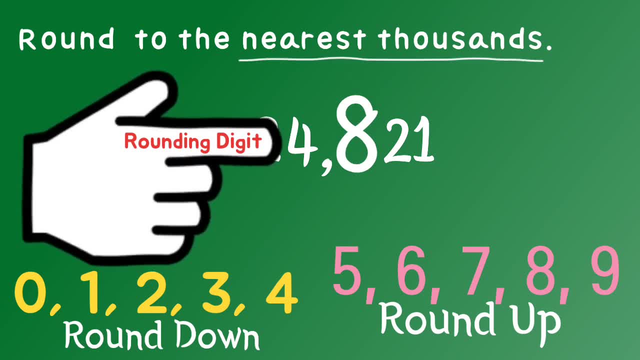 digit. So if this digit to the right of your rounding digit is either 5,, 6,, 7,, 8, or 9, then plus one to the rounding digit, That is roundup- It will become five. Now back to the original roundup. 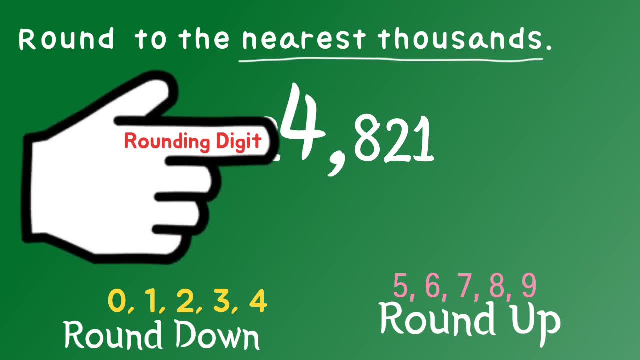 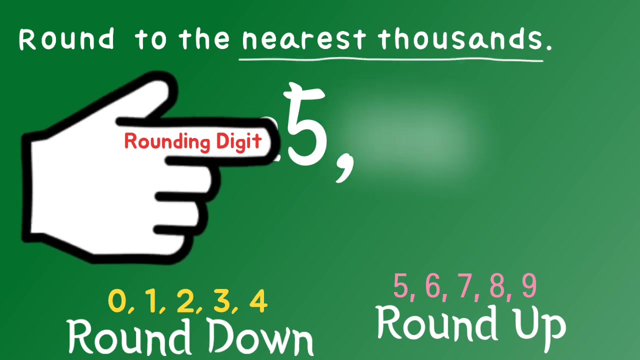 Let's go back to the original roundup. Let's go back to the original rounding digit: Round down or roundup. It is here. so round up Four will become five. Lastly, change all the digits after the rounding digit into zero. So here's 24,821. 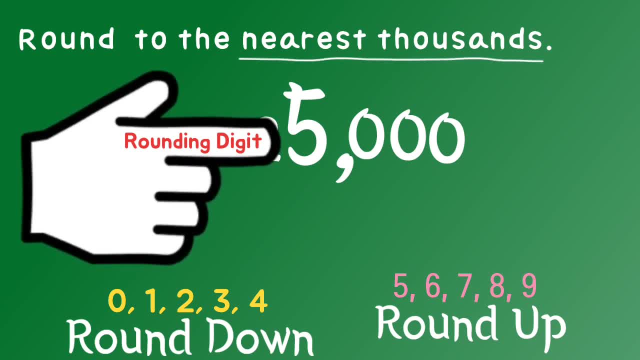 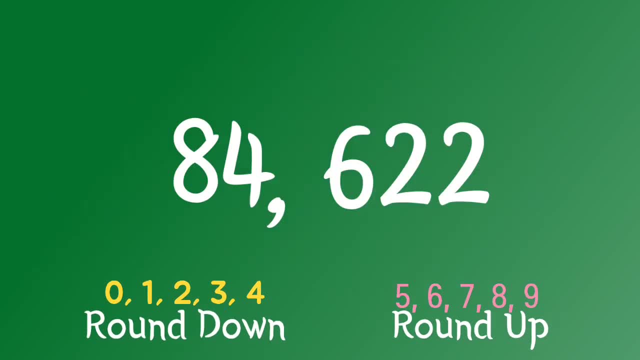 That's four, That's five. One, two, three, four, five, six, seven, eight, nine, ten, eleven, twelve, thirteen, fifteen, fourteen, fifteen, sixteen, seventeen, thirteen, eighteen, nineteen, twenty, twenty, twenty. 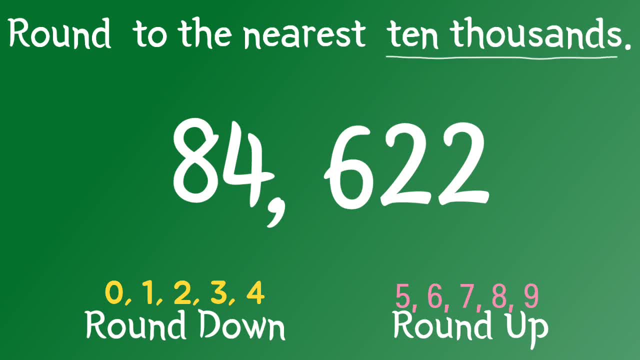 twenty, twenty twenty-nine. One, One, One, One One, Based on the next digit of the rounding digit. you have to decide whether you round up or down. It's here, So round down. Eight will remain eight. 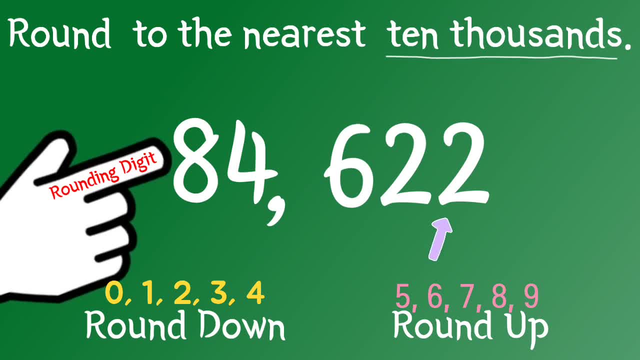 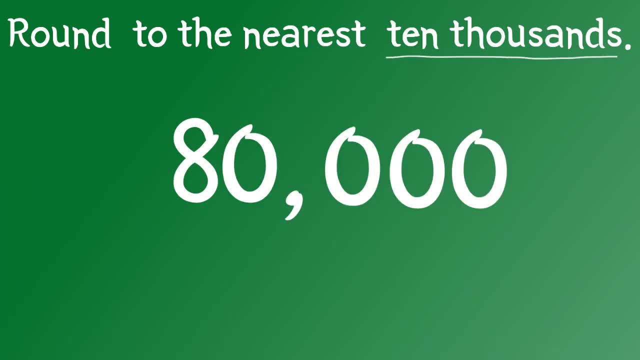 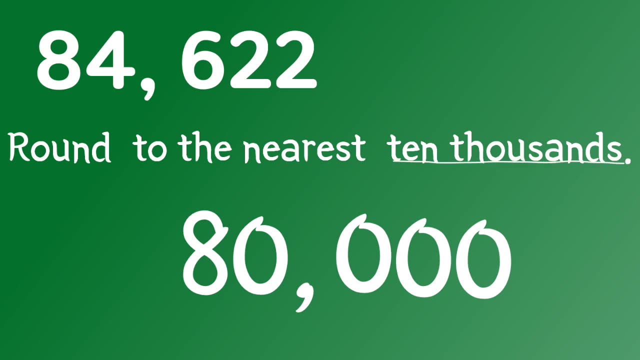 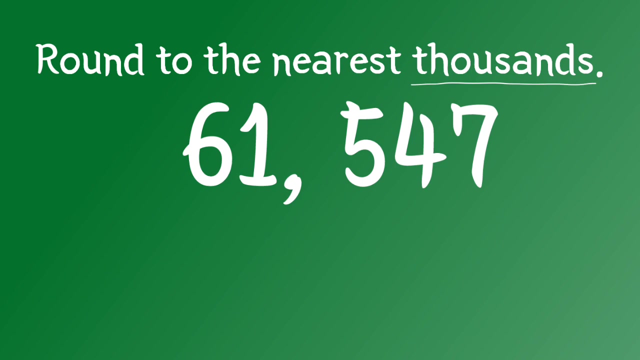 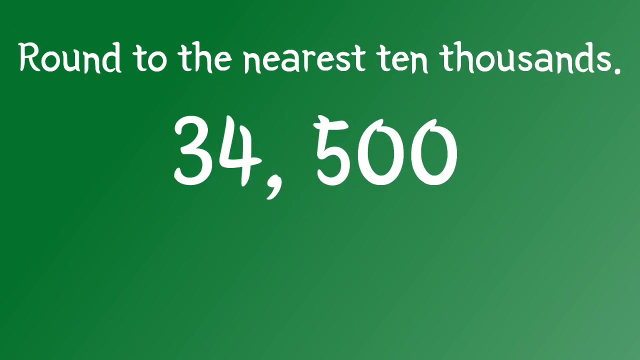 Lastly, change all the digits after the rounding digits into zero: 84,000.. Eighty-four thousand six hundred twenty-two. round to the nearest ten thousandth is eighty thousand. Okay, then try this. What did we do? Step one: